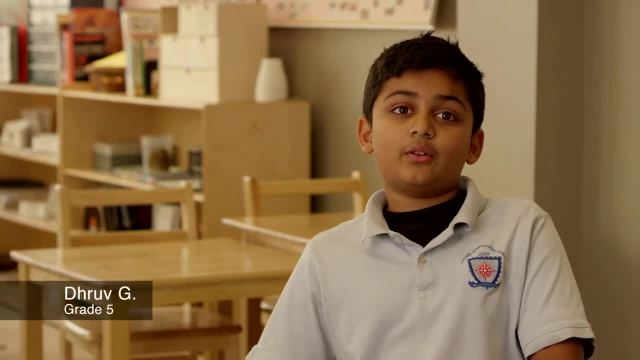 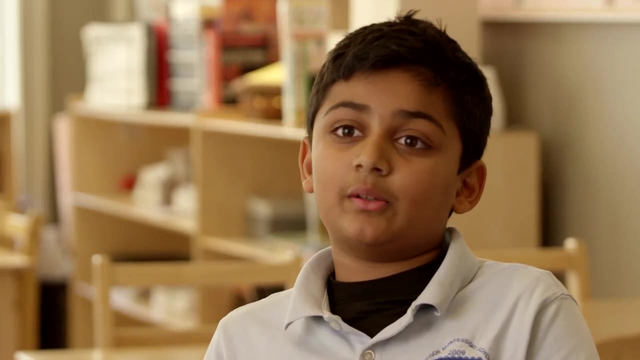 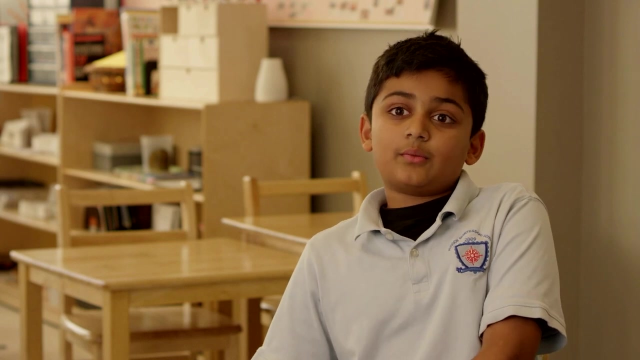 I was most interested about the acids and bases is where you add a hydrogen, for example, like ammonia, It is a base. If you add one more hydrogen, it's ammonium and it becomes an acid And DNA deoxyribonucleic acid. it is what makes up us And we just found out. 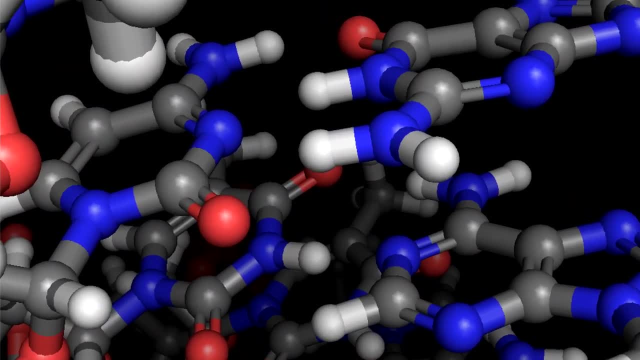 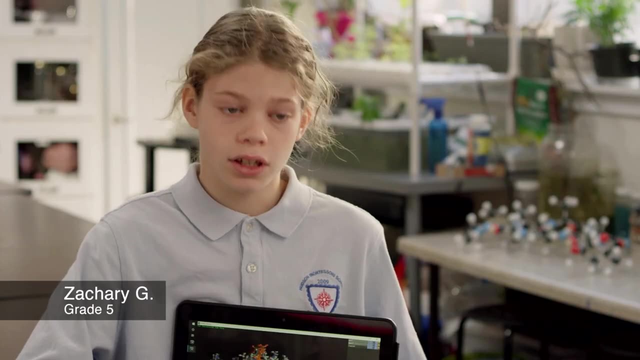 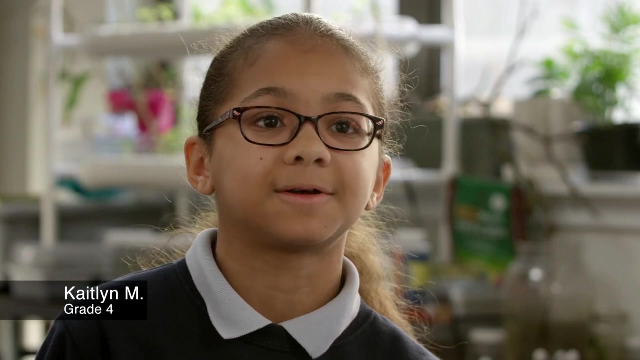 we can actually make it on this thing called Pymol. Pymol is a program that you're able to make molecules and atoms like DNA, like I have right here. You can move it around. It's 3D, You can zoom in and zoom out and do all of that stuff. 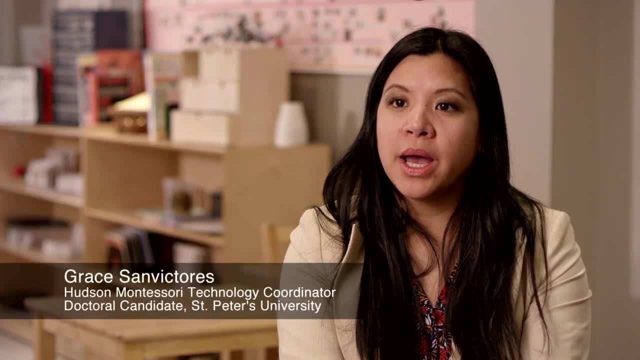 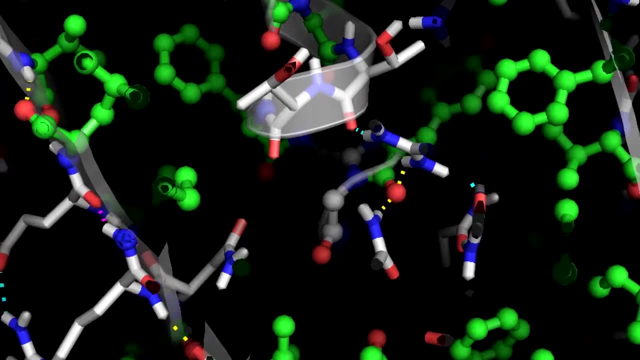 Pymol is a programming software that combines Python and mole for molecules. They see the patterns, They see the sequencing. They're so excited to see a new software introduced to them and they're able to manipulate it with that. They're able to manipulate it with that. 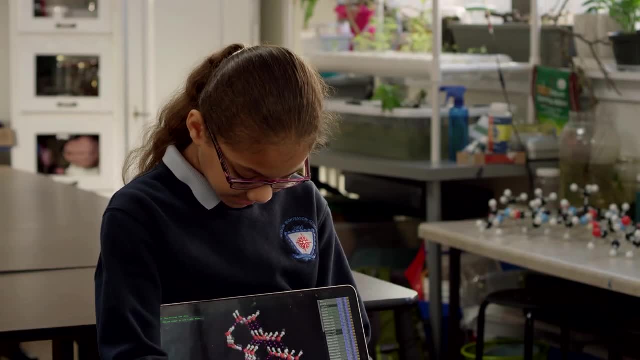 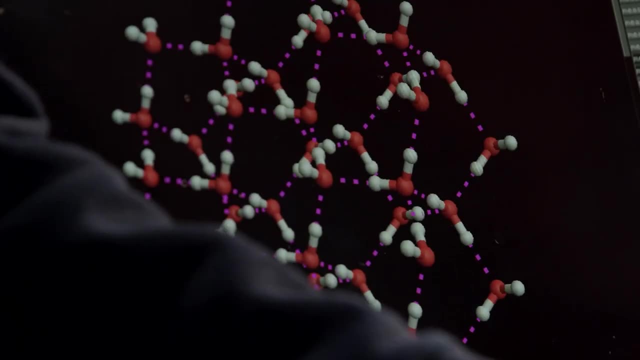 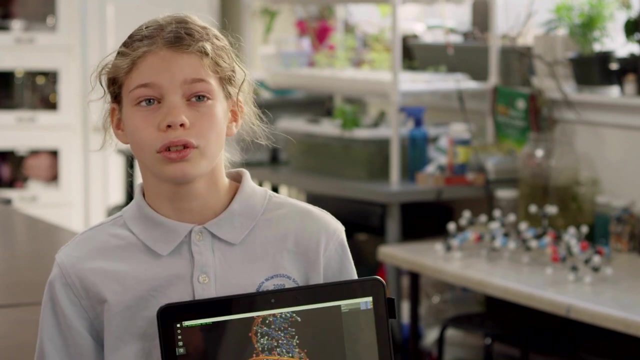 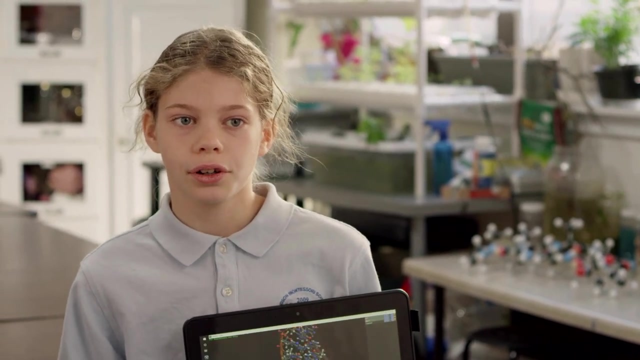 with ease. This is the snowflake model and these are water molecules, and then the like dots are how they connect. It can connect to each other using hydrogen bonds. Hydrogen bond is when you have a lone pair of electrons and it connects to a hydrogen, which makes a hydrogen bond. Well, I think it's a. 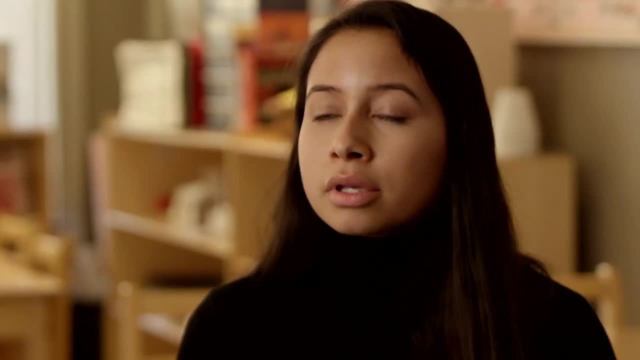 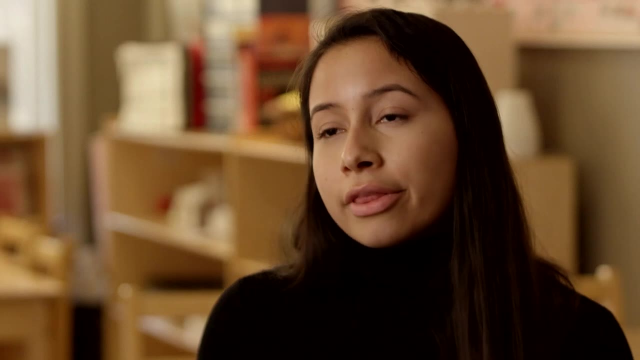 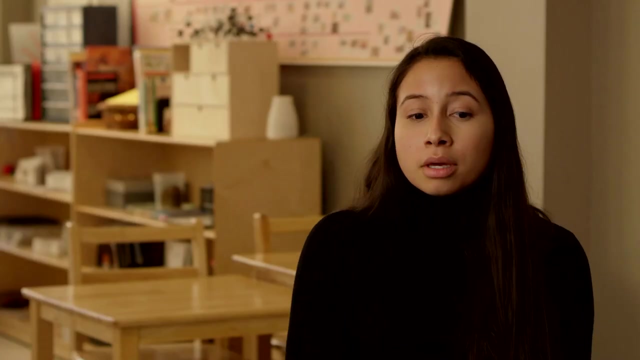 combination of the 3D building molecules, the visual presentations, the pie mold and how. we are not telling them what they're not capable of, but instead we are letting them explore their options and we're letting them build whatever they want and, surprisingly, most of them get it right the first time. 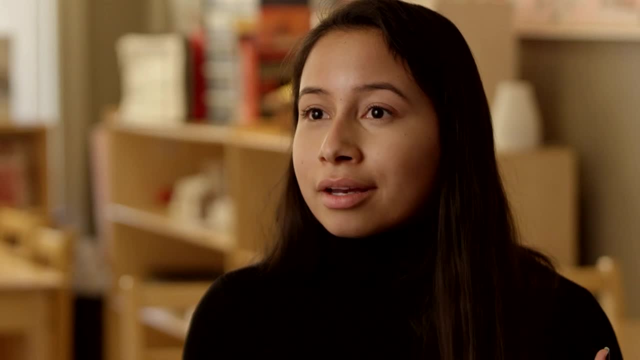 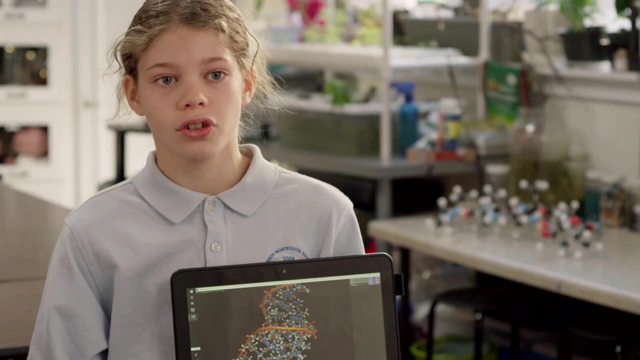 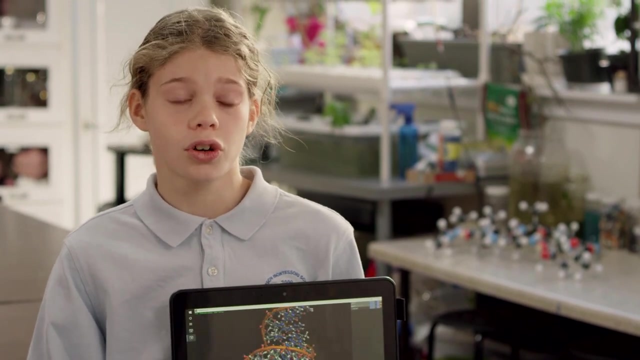 They're building molecules that they don't know, that are capable of being synthesized, and done that way, It's a natural, biological world. so that's really impressive: Nitrogens, oxygens, sulfurs and then carbons, and it runs in all our bodies. 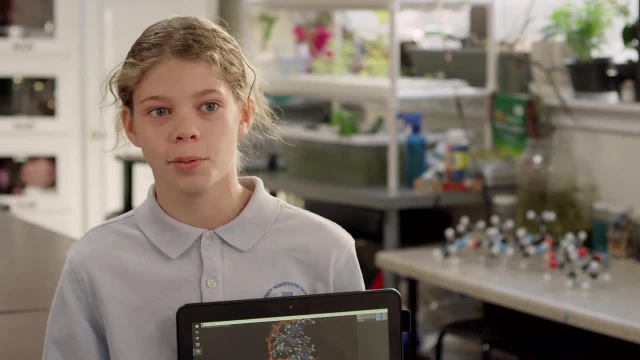 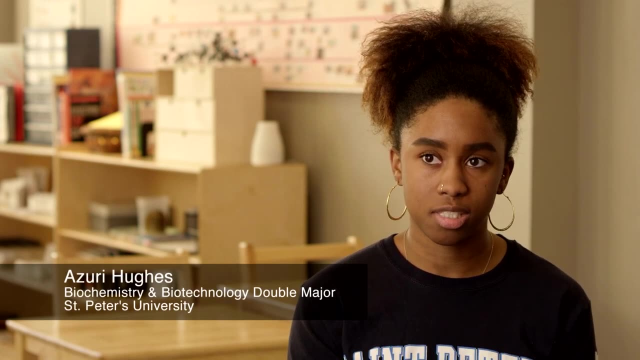 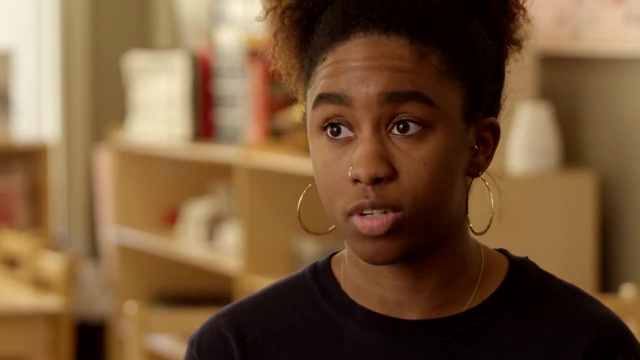 and it once makes a human a human and a pig a pig. If I learned this at a younger age I would probably understand how molecules are in space. When I got to organic chemistry it was kind of hard for me to visualize how molecules look in 3D space. but with the model kit now they know what the molecules actually.